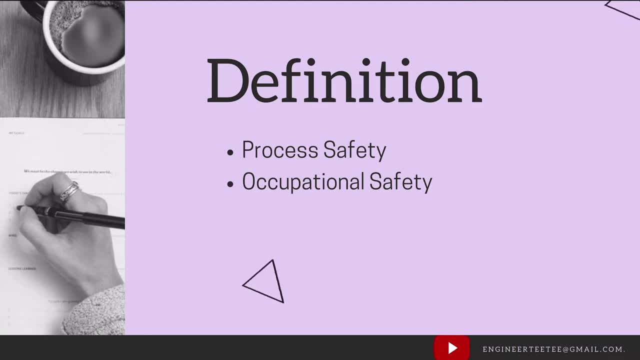 damage to properties, production losses and adverse business publicity. On the other hand, occupational safety deals with all aspects of physical, mental and social health and safety in the workplace. The hazards that fall under occupational safety include slips, trips and falls, exposure to noise, exposure to fires that could cause minor burns and cuts. 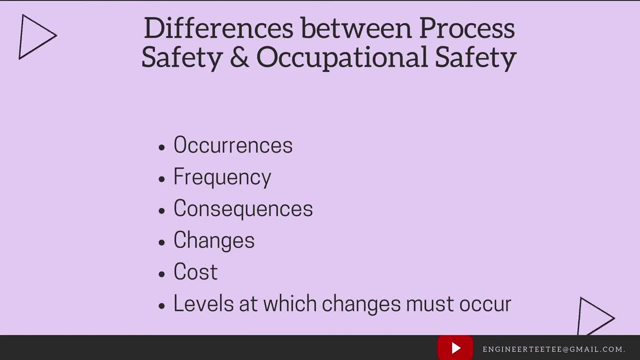 and repetitive strain injuries. Now to the differences between process safety and occupational safety. The first thing is that occupational safety is a process safety. That process safety includes the prevention of unintentional releases of chemicals, energy or other hazardous materials, whilst occupational safety refers to the classic health and safety that is normally associated with the prevention of trips, slips and falls. 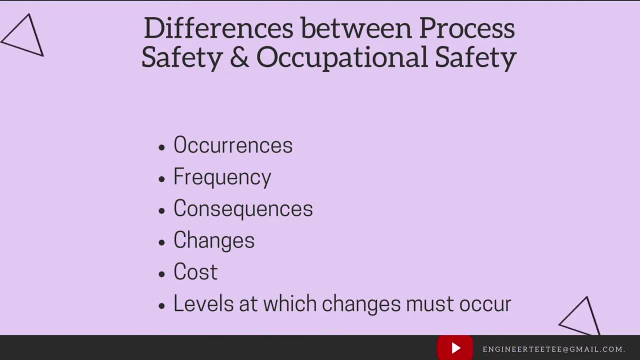 Next we can talk about the frequency Process. safety incidents generally happen at the lower frequency, whilst occupational safety incidences happen at a higher frequency, mainly because these involve human beings, so it's very easy for someone to be walking along and trip if the mitigation measures are not in place. 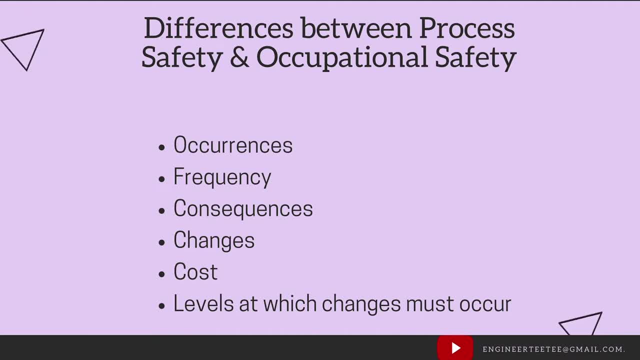 Now. process safety protects workers and public alike, as well as equipment on your chemical plant Whilst. occupational safety protects focuses on the workers. Process safety considers the consequences of accidents at a personal, environmental, equipment and business level, whilst occupational safety focuses on the consequences at human level only. 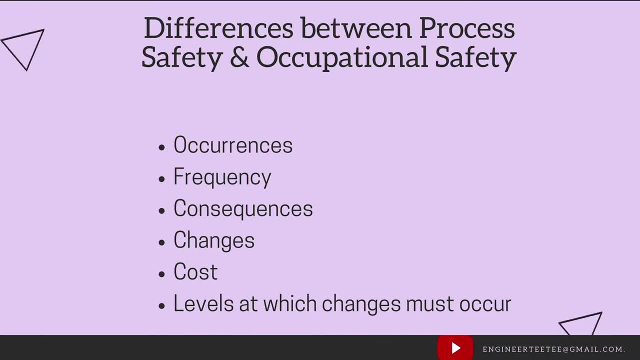 Process safety focuses on changing the system design in which the behavior occurs and elimination of this hazard. Process safety is implemented by engineering design or by providing adequate protection layers, such as safeguards, to minimize the risk associated with the hazard. On the other hand, occupational safety focuses on changing a human being's behavior. 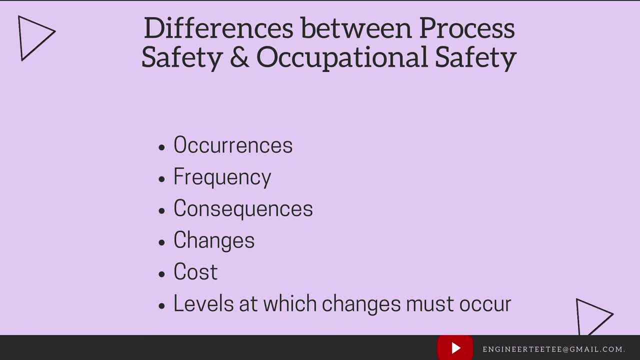 through training and ensuring that people have the adequate personal protection equipment against hazards. Process safety is generally more expensive to implement and is often misunderstood. It addresses major hazards. It targets incidents that are more likely to occur in major incidents with big consequences. Occupational safety addresses incidents involving personal safety at an individual level.